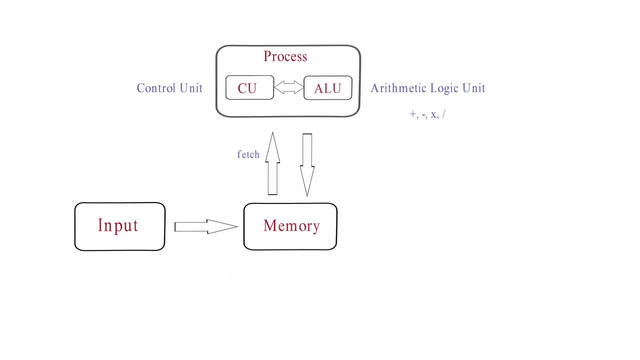 After processing: complete, the control unit stores the result in memory. After processing: complete, the control unit stores the result in memory And display the output. This is the working of von Neumann architecture. von Neumann architecture. Let's discuss components 1. Input. 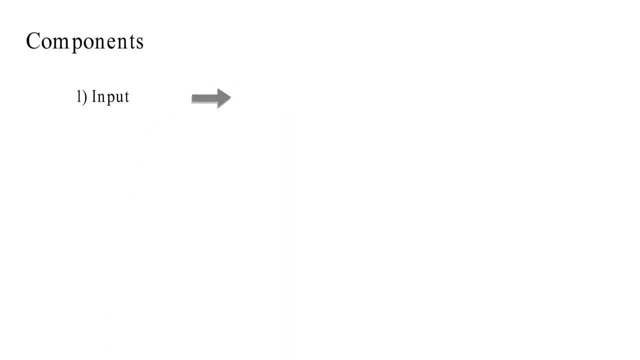 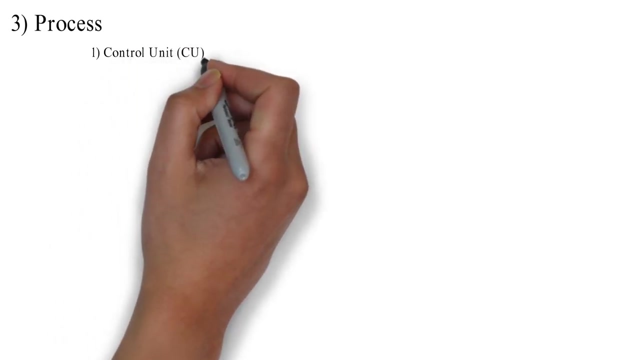 1. Input: Input comes through input device like Keyboard Mouse etc. Keyboard Mouse etc. 2. Memory: The data temporary store in the memory called RAM. 3. Process: Process has two parts: 1. Control unit: The control units works like traffic cop. 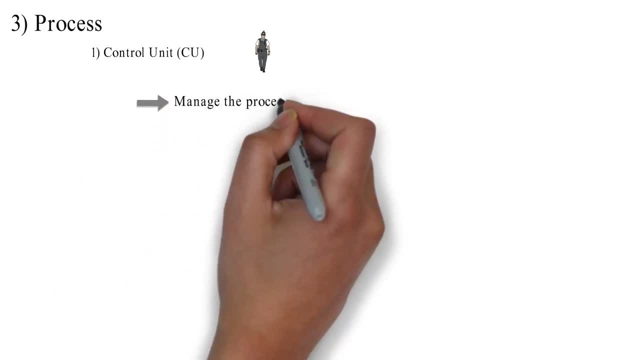 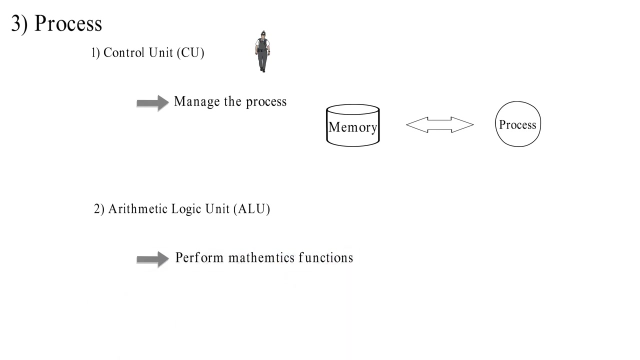 It control and manage the process and input output. The control unit fetch and store data to and from memory. 2. Arithmetic logic unit. The role of the ALU is to perform mathematics calculation, Like addition, subtraction, multiplication, division, etc. 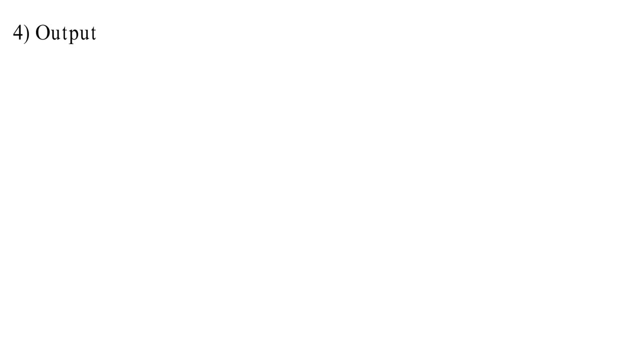 4. Output- The output display through the monitor, printer, etc. We will learn the working of hardware later in detail. Let's understand von Neumann architecture with example. We enter 20 plus 20 through keyboard. The data is stored in the memory called RAM and ready to process. 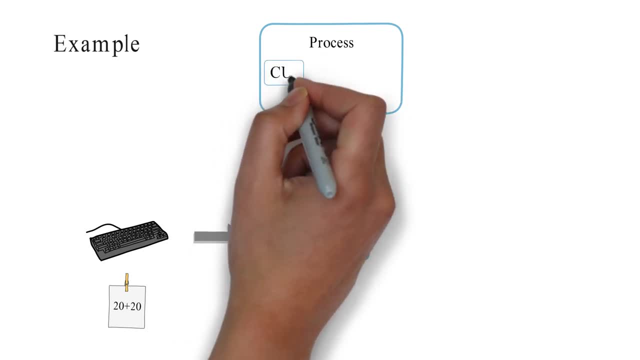 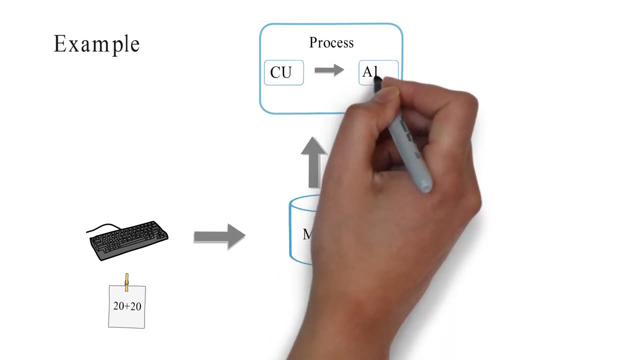 The control unit fetch the command and checks which operation is to be paroform. If it is arithmetic operation, the CU command to the ALU. for operation: ALU perform the operation. Be sure to confirm the addition and send back the result to the CU. 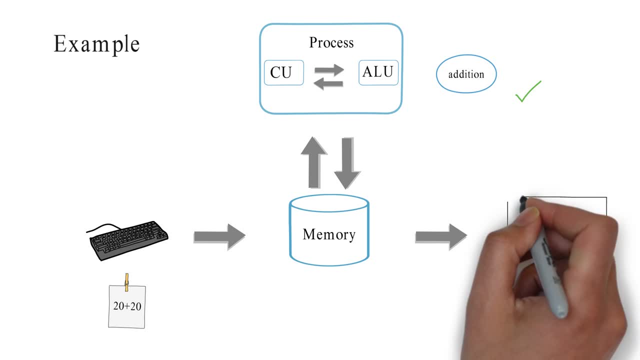 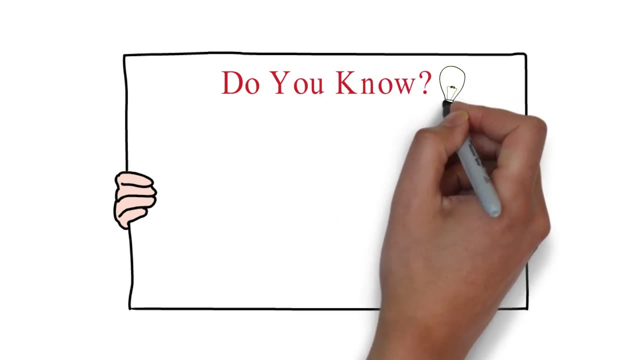 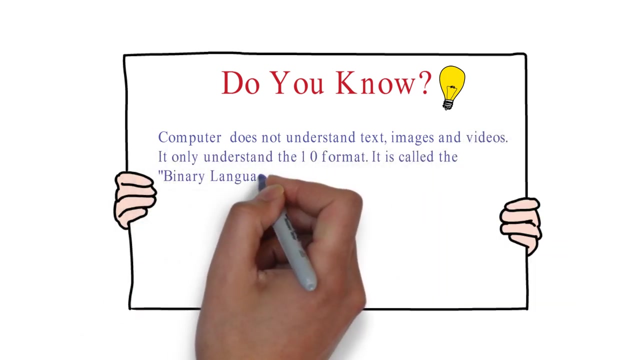 CU store the result in memory and display it through output device. Do you know? Computer does not understand text, images and videos, It only understand the look Н forms. It is called the binary language. Computer converted all the text, images and videos inside the display. 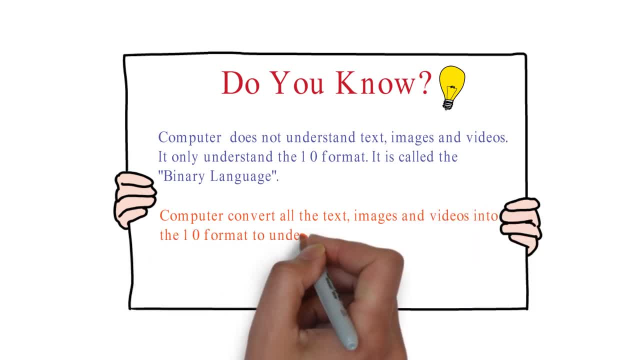 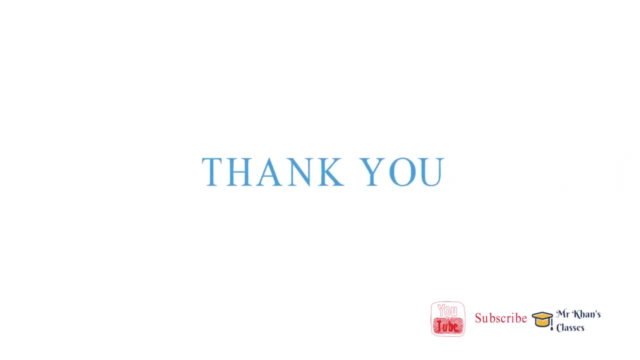 Computer converts other images and videos Located into PNG images and videos into the 1.0 format to understand it.